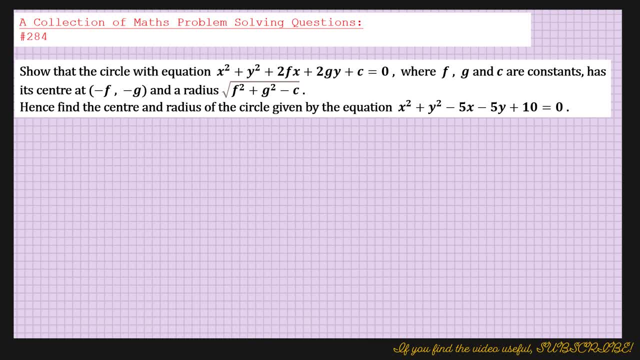 Hence find the centre and radius of the circle given by the equation x square plus y square minus 5x minus 5y plus 10 equals 0.. So the first thing we need to do is arrange the equation we've been given into a format which represents the equation of the circle. 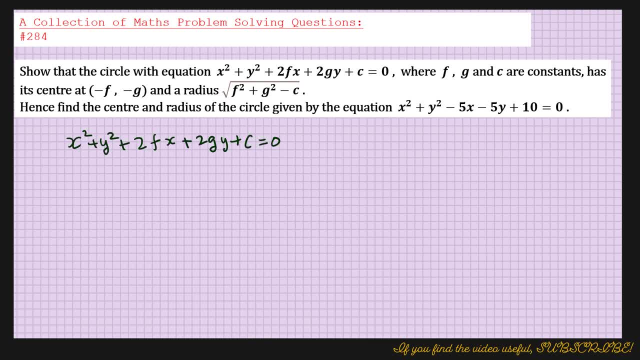 Now we can do that By grouping together the x square and x terms and the y terms, So we would get x square plus 2fx within the bracket and plus y square plus 2gy, and then keep c separate, And then we can try and write it as the sum of two squares. 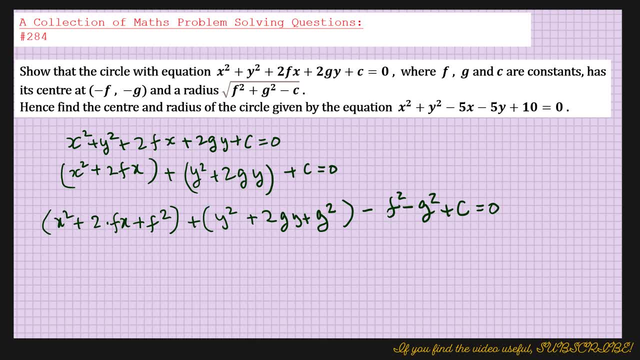 So we're going to do x square Plus 2fx plus f square, and with the next one we do y square plus 2gy plus g square. So what we are trying to do is write it in the form x plus f whole square and y plus g whole square. 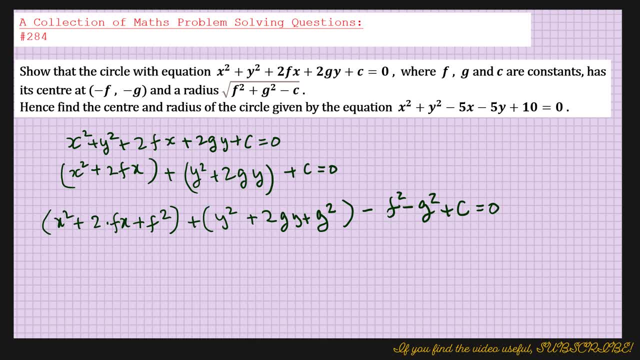 And then, because we have introduced two new terms, f square and g square, we've got to subtract them. That's what we do: minus f square minus g square plus c. So then it can be written as x plus f whole square, plus y plus g whole square equals f square plus g square minus c. 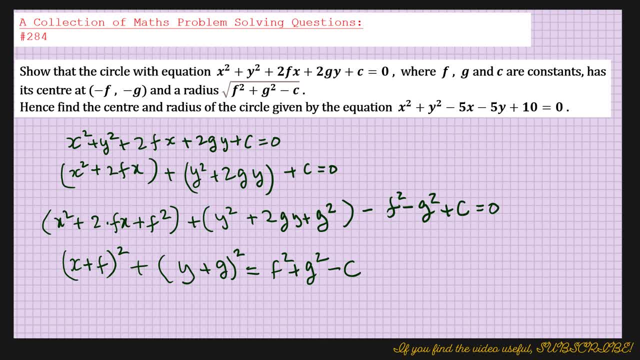 And you see, this is very much in line with the equation of a circle. Because the equation of a circle can be written as: x minus a whole square plus y minus b whole square equals r square. Of course, in this case, if f, a would be minus f and b would be minus g, 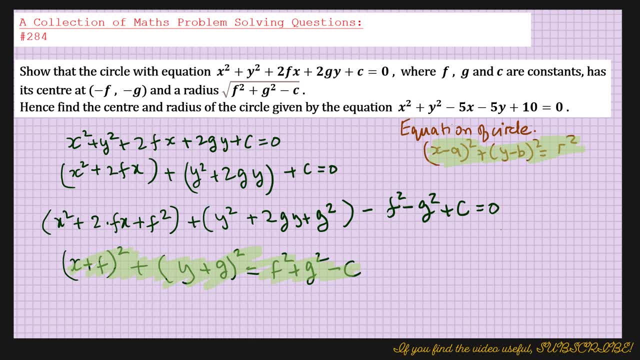 So that is in the format of the equation of the circle with centre a. Now for our x minus a whole square plus y minus b whole square equals r square. The centre of the circle would be ab and the radius would be r, And so that's. 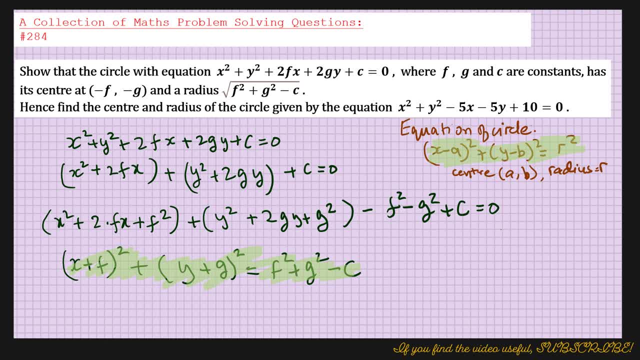 That's done. I mean yeah For the equation that they've given us. so x plus f, whole square. Now if you see what is going to be the centre, it's going to be obviously minus f, Because here you are having plus f. 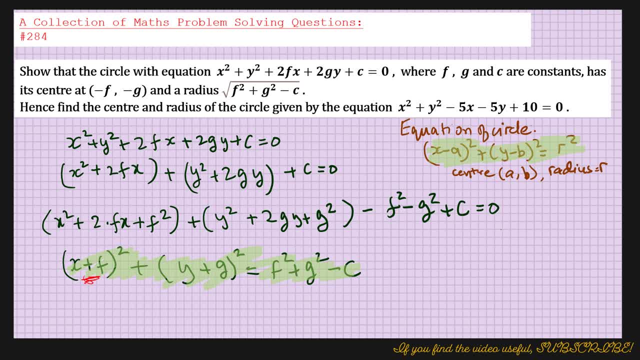 So obviously, to make it same as the standard equation, this has to be minus f, So it's the radius. Sorry, the centre has to be at minus f and minus g. So we write: centre is minus f, minus g And the radius has to be the square root of f, square plus g, square minus c. 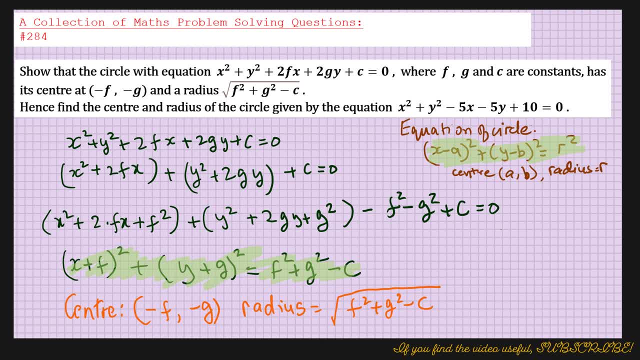 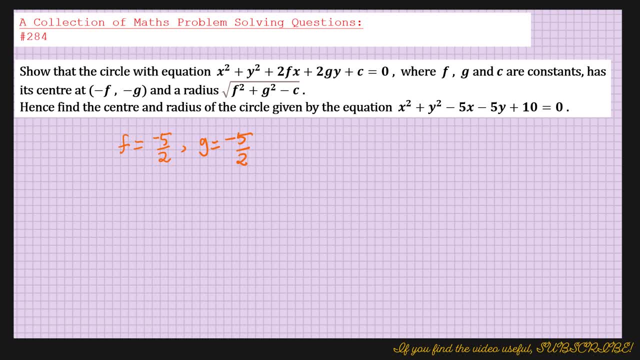 So that completes the first part of the question. For the second part, all we have to do is We have to Look at the equation, the standard equation of the circle, And we have to find out and have to, You know, we have to find the term. 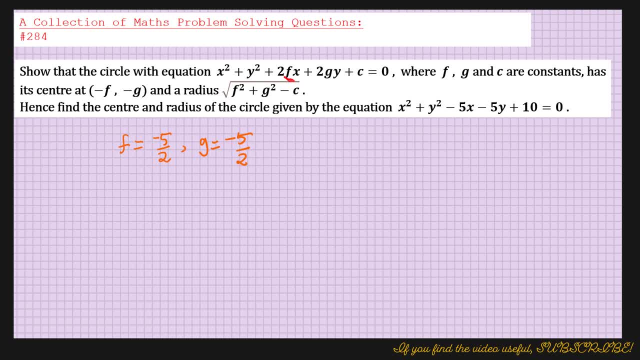 So f here would equal What? twice of f here is minus 5.. And twice of g is also minus 5.. So therefore, f would be minus 5 out of 2. And g would Would be minus 5 out of 2 as well. 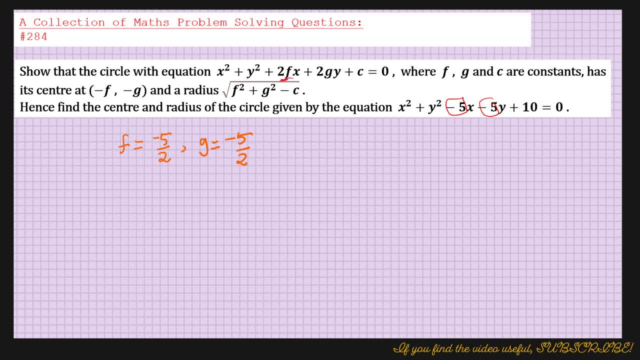 So this is what it is, And it is 2g. So that's what it is. That's the centre of the circle, And then we need to find the radius. To find the radius, so you have This is f or twice of f. 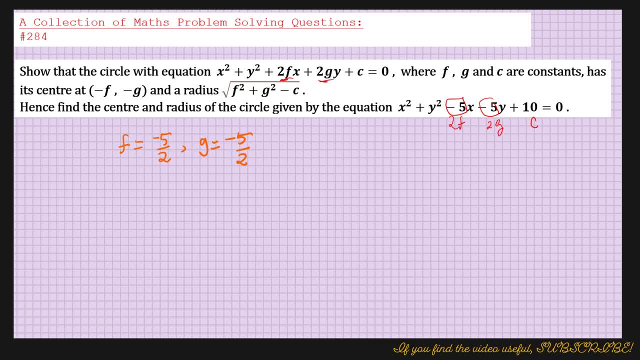 And this is twice of g And this is your c. So the radius of the circle would be Minus 5 out of 2.. 2 whole square plus And then minus 5 out of 2 whole square And minus 10.. 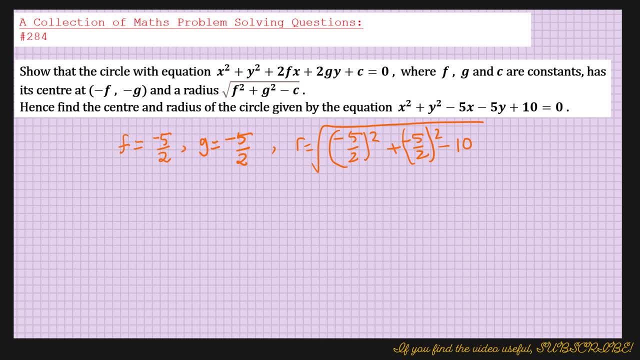 That is the radius. So we just substitute the values And we get radius equals square root of 10 divided by 2.. So I think we've answered all the parts to the question And that completes it. Thank you very much for watching. 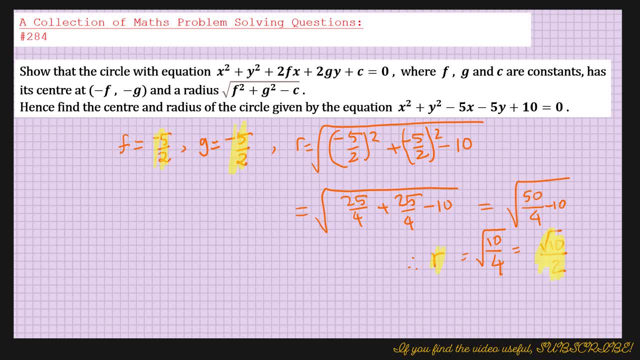 I hope you enjoyed this video And I will see you in the next video. Bye, bye.